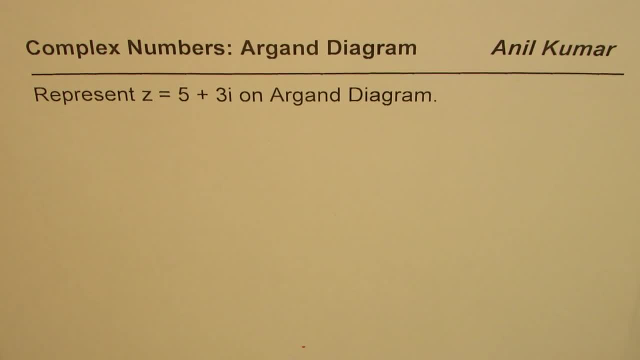 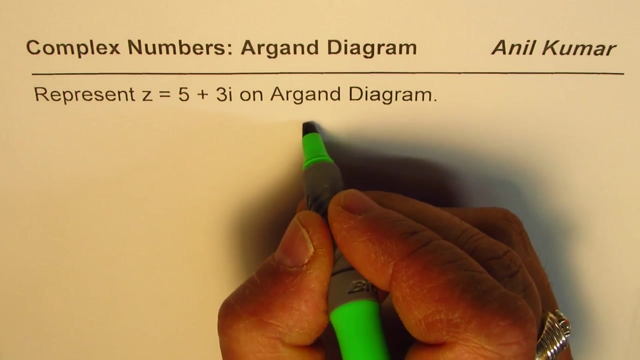 I am Madhul Kumar and in this video we will learn how to represent complex numbers in the form of a diagram. Question here is: represent z equals to 5 plus 3i on Argan diagram? Now, Argan diagrams are the diagrams where the vertical axis represents the imaginary numbers. 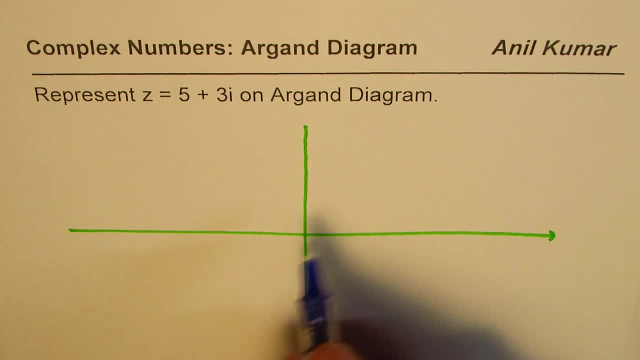 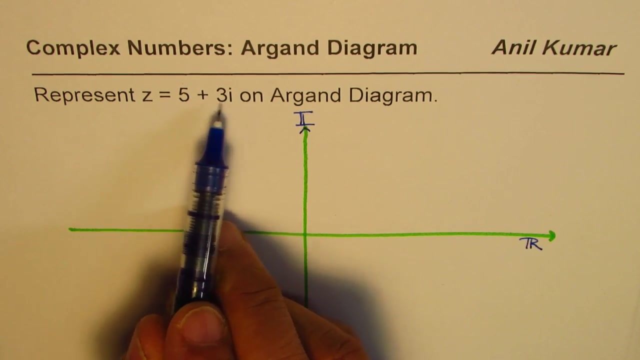 the horizontal axis represents the real numbers, right. So the horizontal axis will write the real numbers and the imaginary numbers will be represented on the vertical axis. We need to represent the complex number. z equals to 5 plus 3i. Now 5 is the real part and 3 is a coefficient of imaginary part, right. 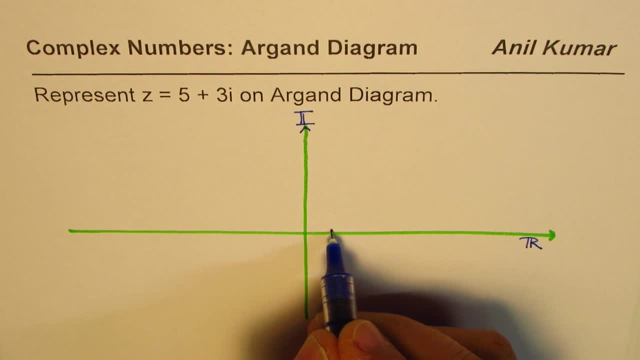 So let's say, let's write marks like 1,, 2,, 3,, 4,, 5, right? So this is like 1 for us, So this is 4.. This is 5.. That's on the real side. 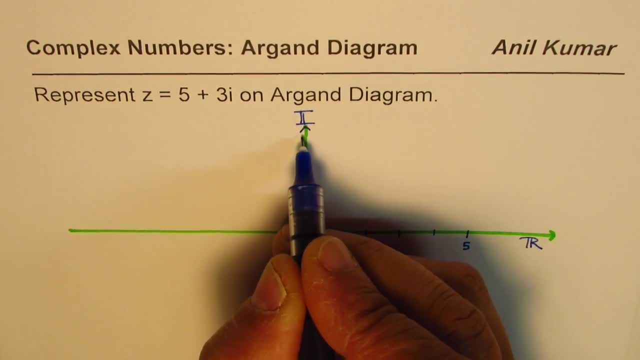 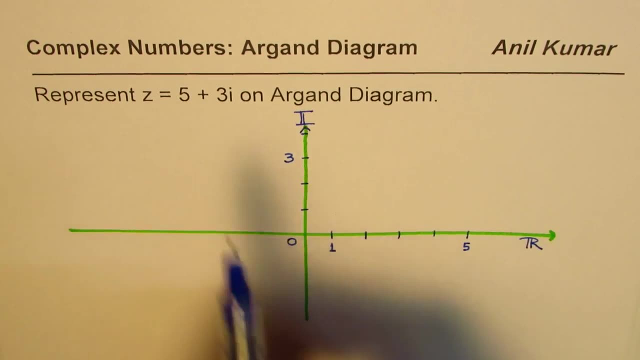 On the imaginary side. let's say 1,, 2,, 3,, 4.. So this mark is third And this is the 0 for us, correct? So 5 plus 3i will be. we have to move 5 units towards the real side. 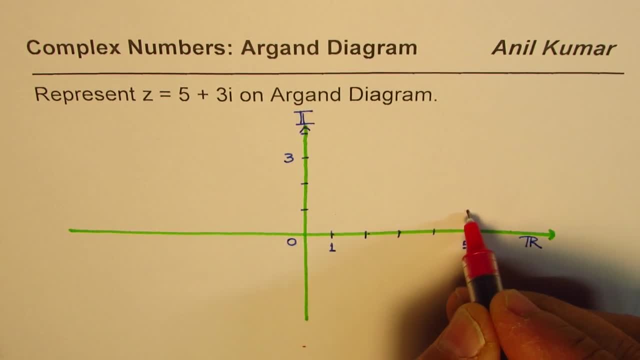 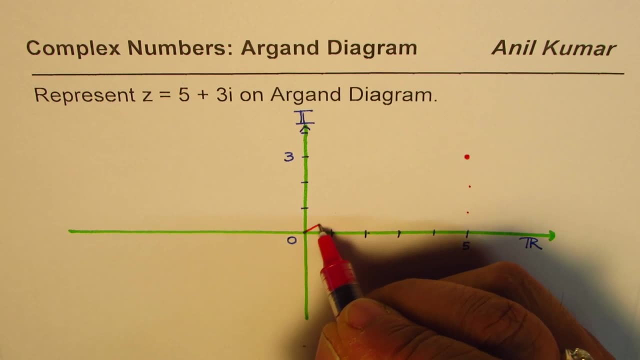 So 1,, 2,, 3,, 4, 5, and then go 3 up, 1,, 2 and 3.. So this point here represents the complex number. So this is how we could do it right. 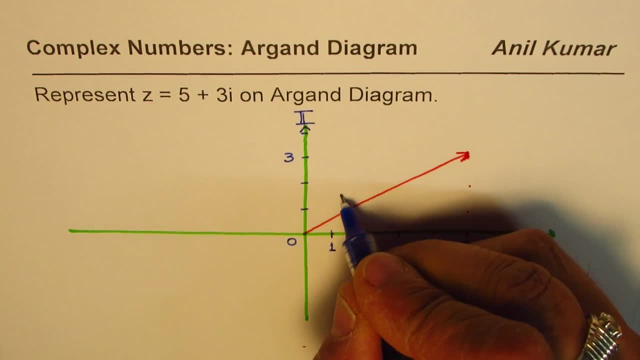 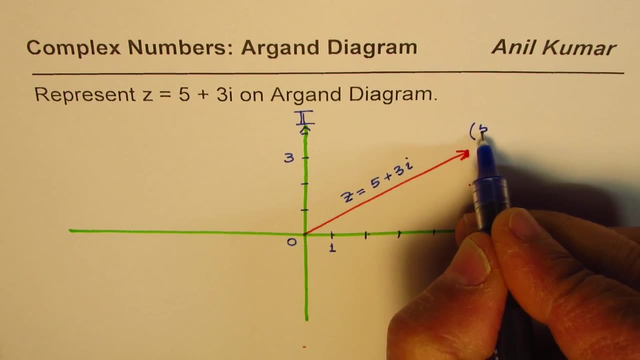 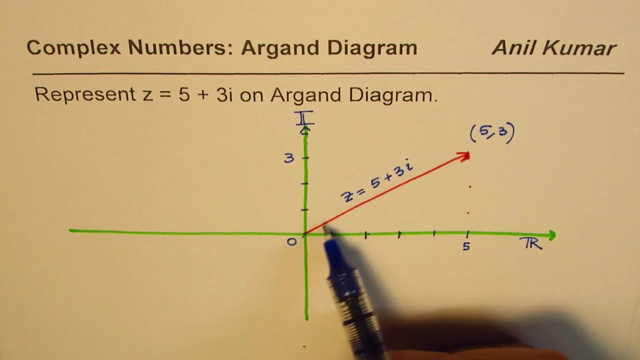 So this point here represents z, which is equals to 5 plus 3i, right. So in rectangular coordinate we can also write this as 5 comma 3.. Is that okay? So that is how you can represent The magnitude of this. represents 5 square plus 3 square square root. 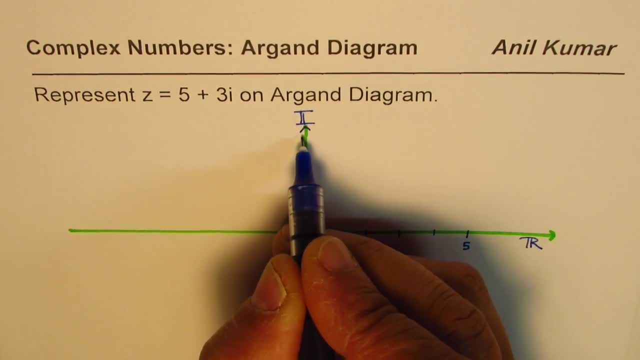 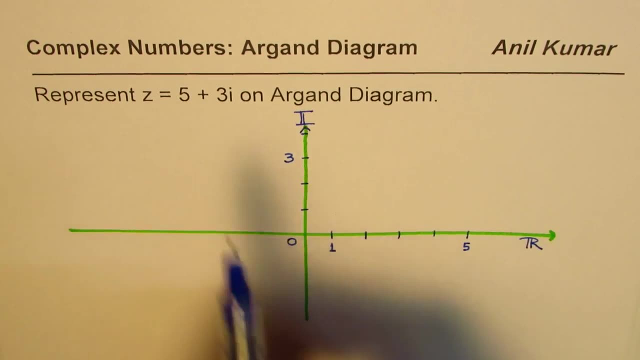 On the imaginary side. let's say 1,, 2,, 3,, 4.. So this mark is third And this is the 0 for us, correct? So 5 plus 3i will be. we have to move 5 units towards the real side. 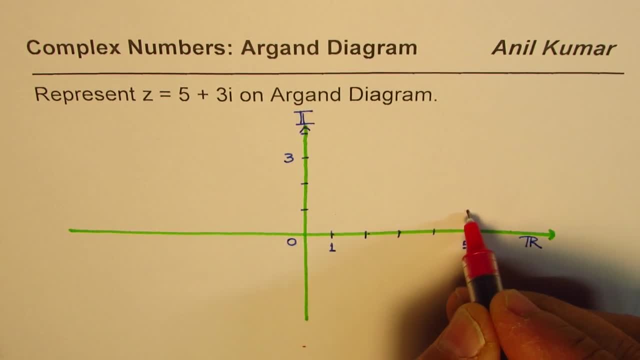 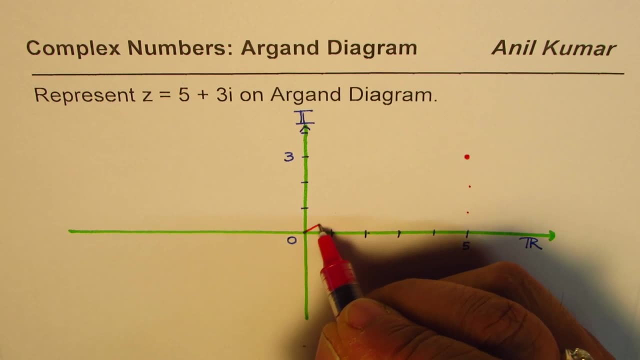 So 1,, 2,, 3,, 4, 5, and then go 3 up, 1,, 2 and 3.. So this point here represents the complex number. So this is how we could do it right. 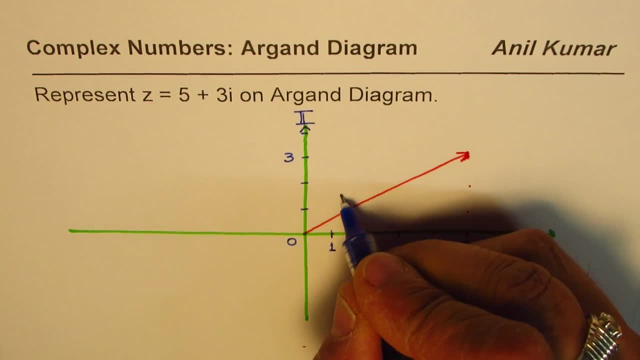 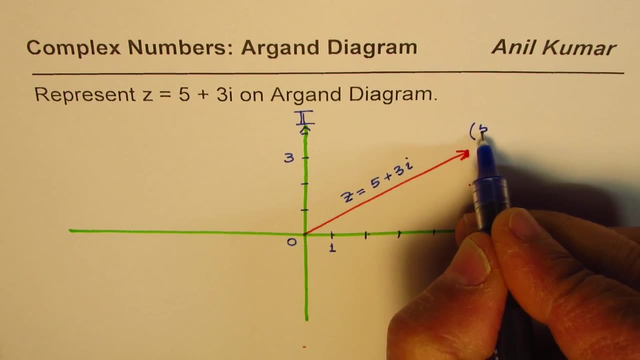 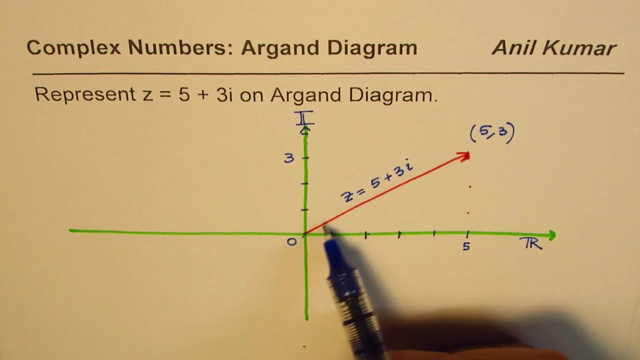 So this point here represents z, which is equals to 5 plus 3i, right. So in rectangular coordinate we can also write this as 5 comma 3.. Is that okay? So that is how you can represent The magnitude of this. represents 5 square plus 3 square square root. 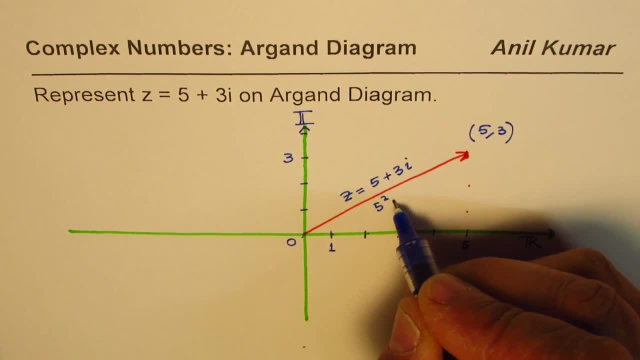 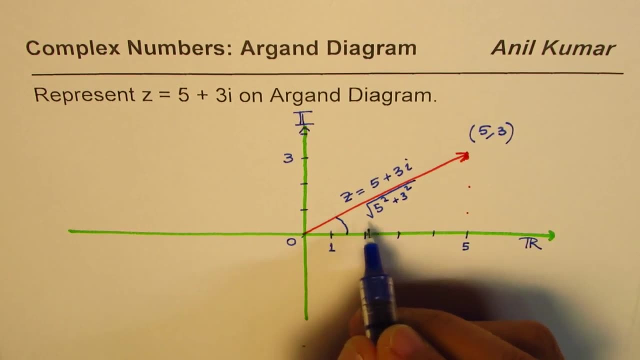 So this length will be equal to 0. This is equal to 5 square plus 3 square square, root right. And we can actually find the angle also right- Which is not required Anyway- by finding the theta. Let's say: this is the angle phi. 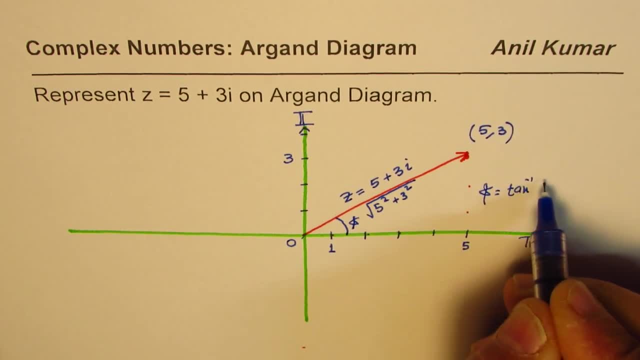 We could actually find the angle phi as tan inverse of the real and imaginary power ratio, which is 3.. The vertical side over phi, right? So that's another thing. But anyway, if I write r and theta, that'll be in the polar form, correct? 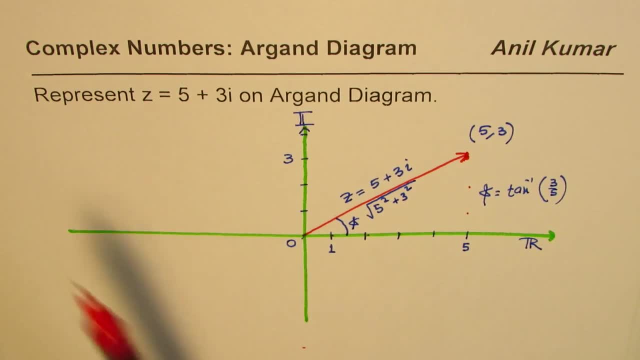 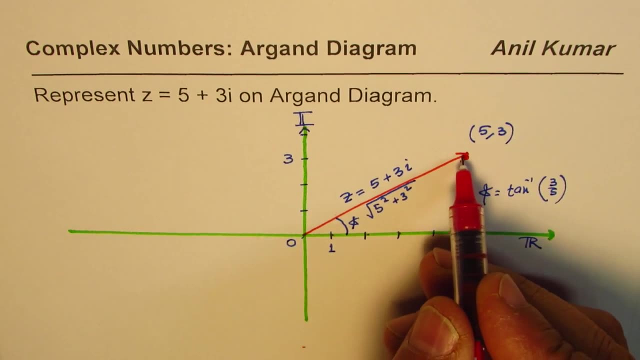 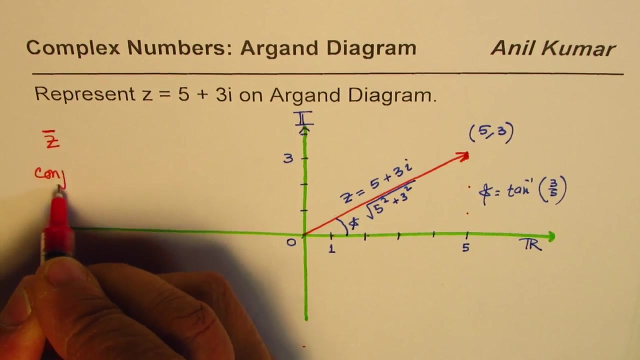 We're not getting them there, But this is how you could represent the complex number 5 plus 3i. Now a question for you. So we already have the complex number z. How will you represent the conjugate? How will you represent the conjugate? 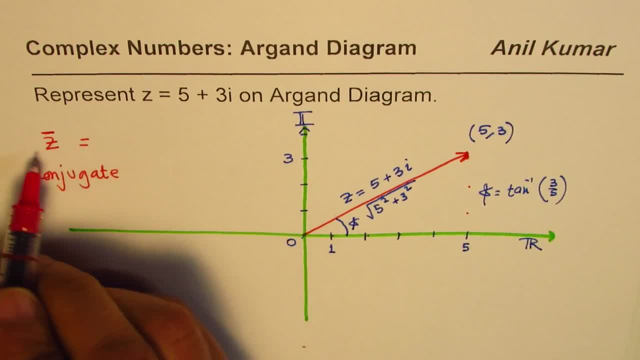 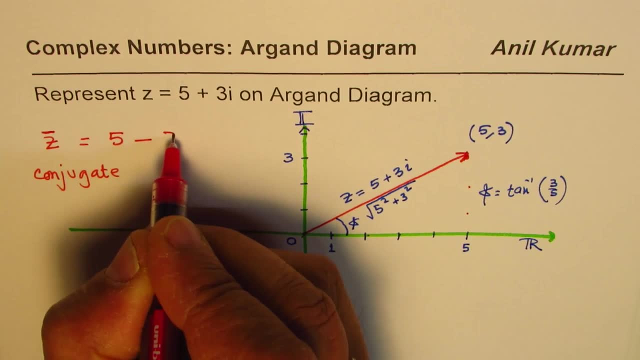 Can you answer me that? So how will you represent conjugate of this complex number? Conjugate is the sign changes. It becomes 5 minus 3i, Is that okay? So what will happen? So conjugate, you see, it is 5.. 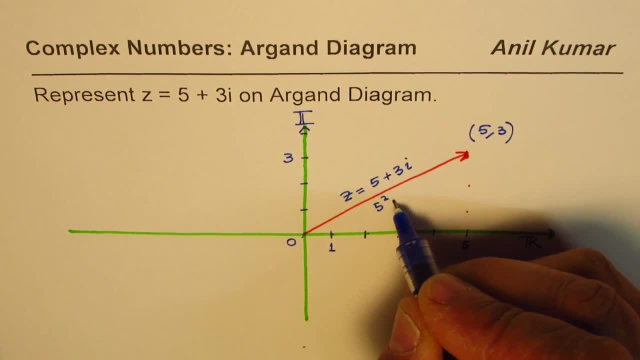 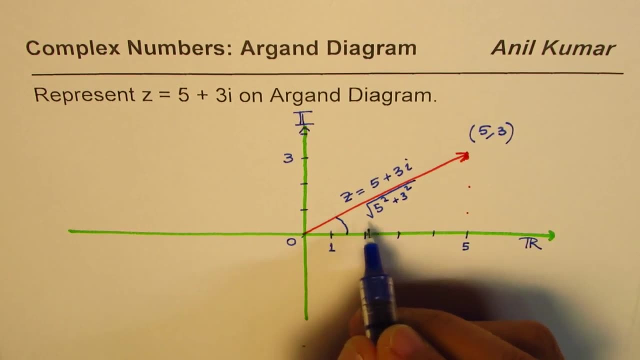 So this length will be equal to 0. This is equal to 5 square plus 3 square square, root right. And we can actually find the angle also right- Which is not required Anyway- by finding the theta. Let's say: this is the angle phi.